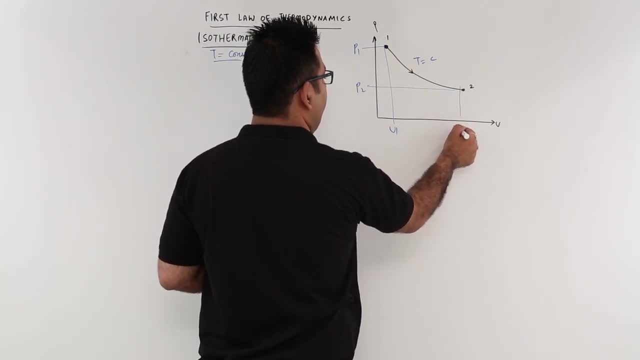 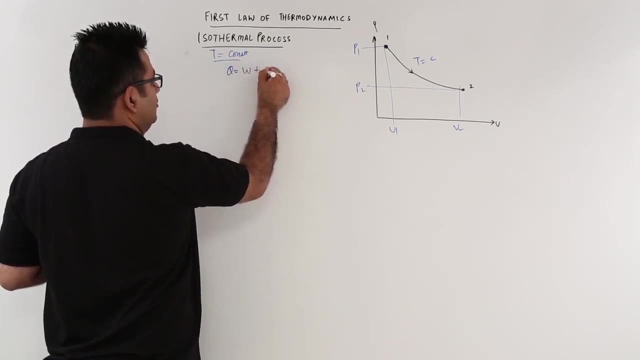 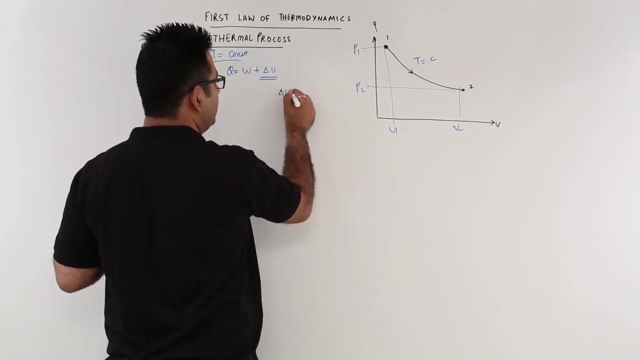 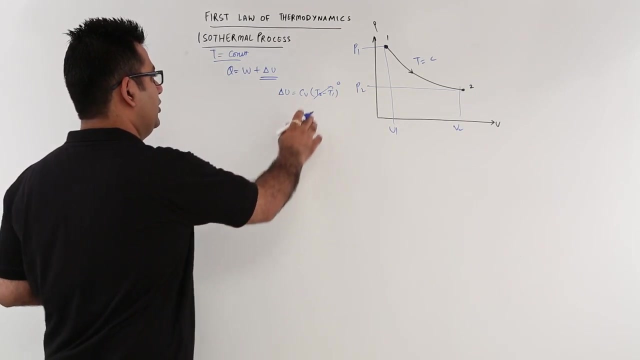 So you have P1, P2, V1 and V2.. So if you apply the first law, because the temperature remains constant, so we know that delta U is equal to Cv into T2 minus T1. Now T2 minus T1 is a zero value because both the temperatures are same. 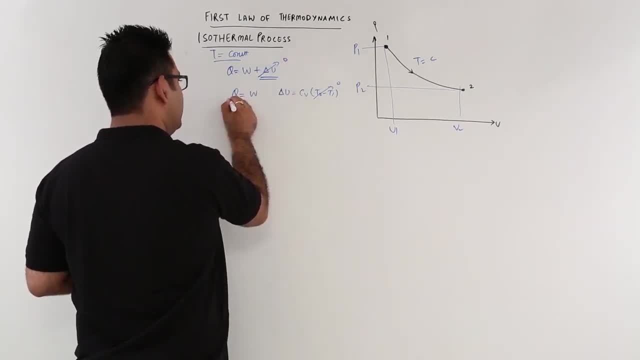 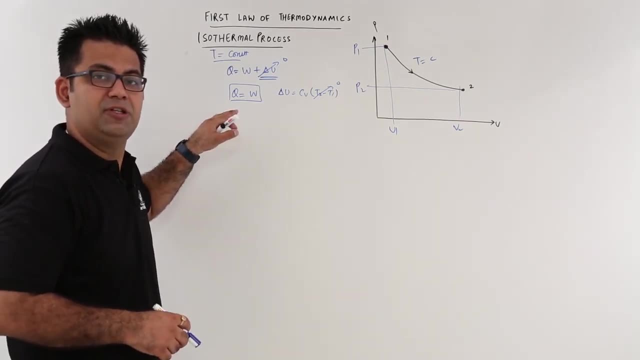 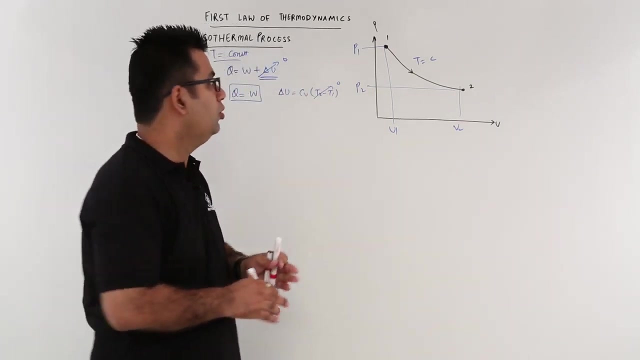 So delta U becomes zero. So whatever heat you supply gets converted into equal amount of work. Now, this is not. This is not possible. This is an impossible mathematical relation. So this means that this process is an hypothetical process. You do not have isothermal processes occurring in nature in actuality. 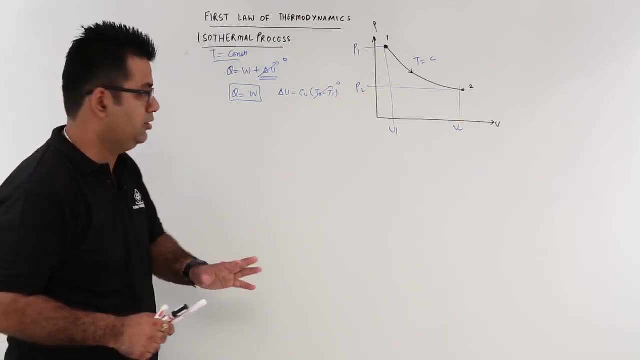 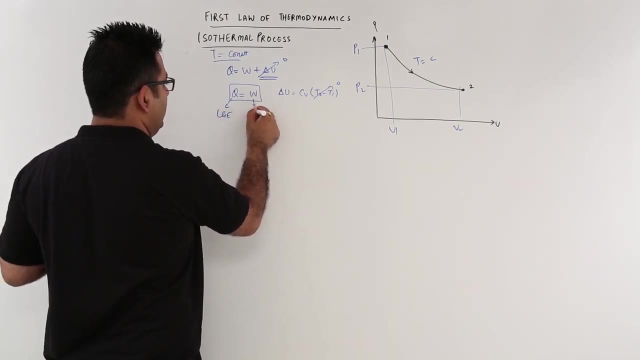 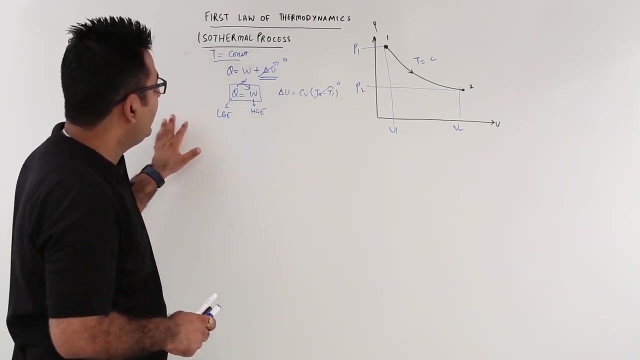 Because Q is equal to W is not completely possible because Q is a low grade energy and W is high grade energy, So the complete conversion is not possible. Okay, Now, if you find out the value for W. that is the work done in an isothermal process. 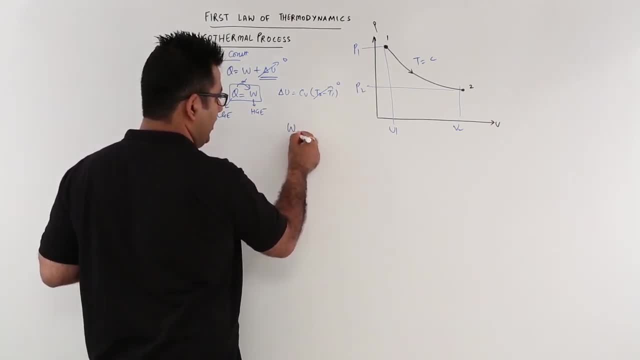 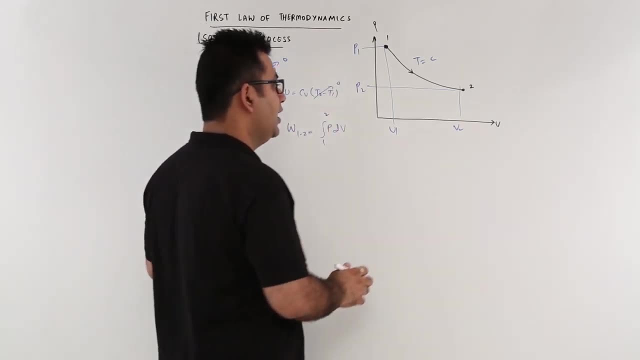 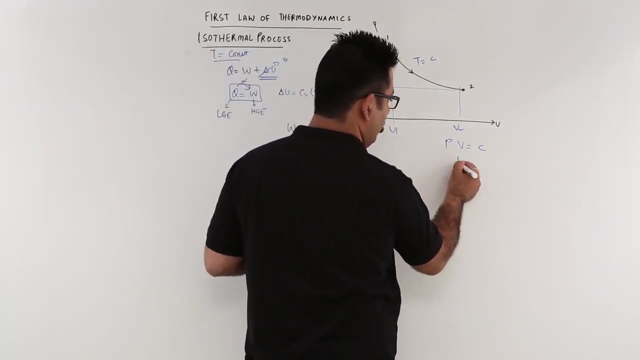 Let us find that out. So work in going from 1 to 2 is PdV. Okay, The mathematical relation is: Pv is equal to constant, because Rt will be a constant. So P is equal to C upon V. Okay, P is equal to C upon V. 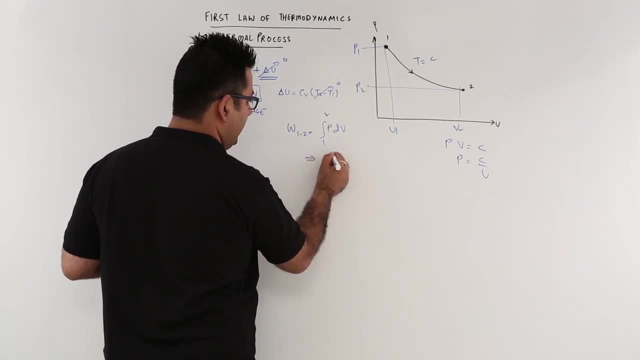 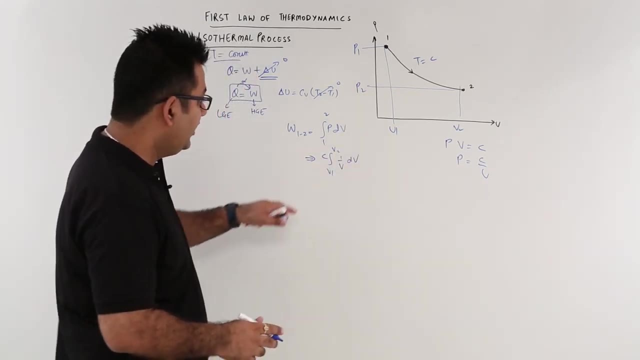 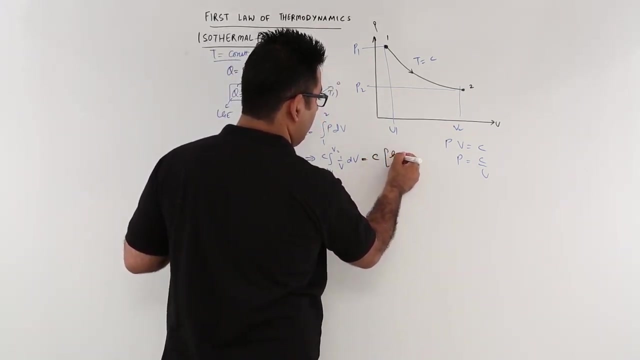 So let us put that over here. So in place of P I can put down C and this becomes 1 over V into Tv. So when you integrate this, this becomes natural log of V. So this is C into natural log of V, V1 to V2.. 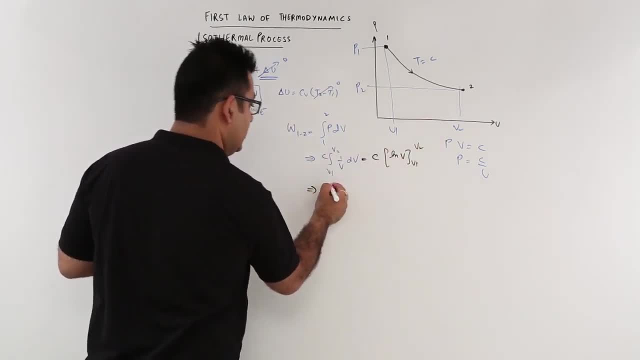 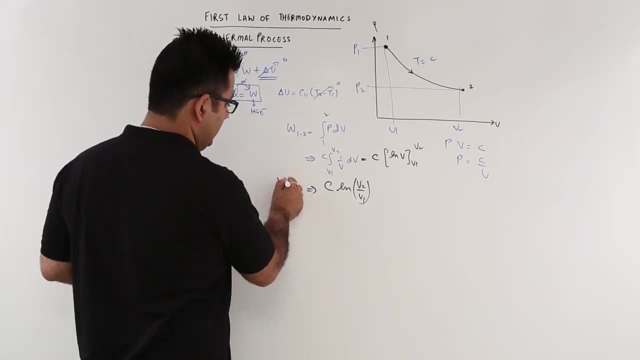 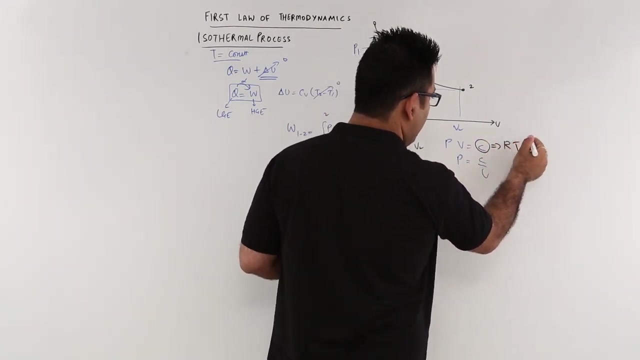 So when you put those limits in place, you get This value Okay, And this is work 1 to 2.. Now, if you look at this, this is nothing but R into T, Isn't it? So you put Rt over here.